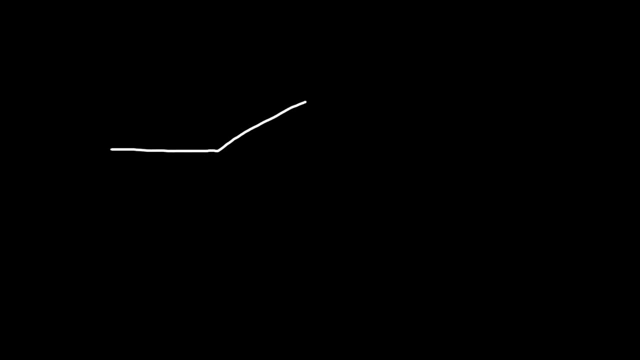 In this lesson we're going to talk about how to calculate the surface area of a rectangular prism. So let me draw a picture first. So let's say this is 12 inches and this side is 5 inches and this is 3 inches. 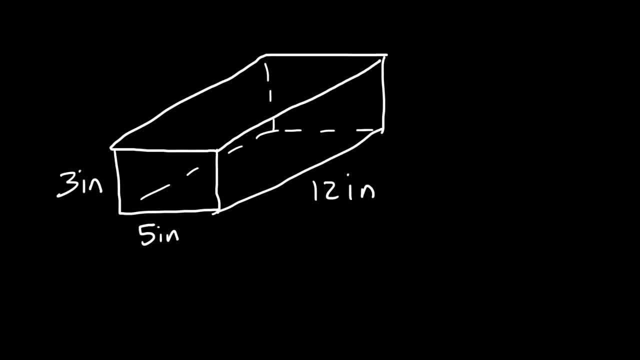 What is the area of this rectangular prism? the total surface area. So let's come up with an equation. first We need to calculate the area of all six faces. So let's call this ABCD and let's say this is EFGH. 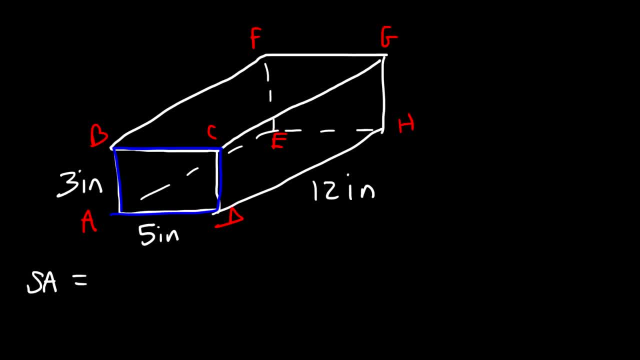 So first let's calculate the area of ABCD and EFGH, So those two faces. they have a width of W and a height H, So the area is going to be W times H And because there's two of them, it's going to be 2WH. 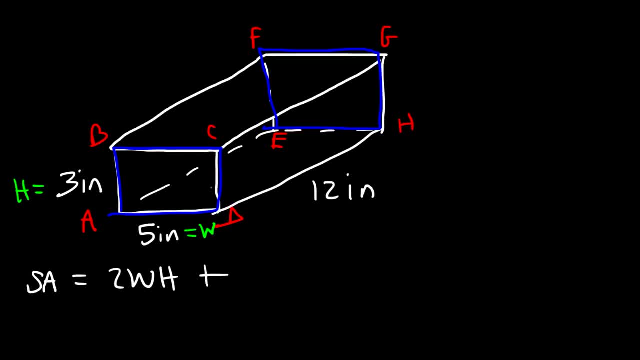 And then we have the face on the right, let's say CDHG, and then the one on the left, ABFE. So those two faces, they have a left L and also a height H, So the area is going to be 2LH. 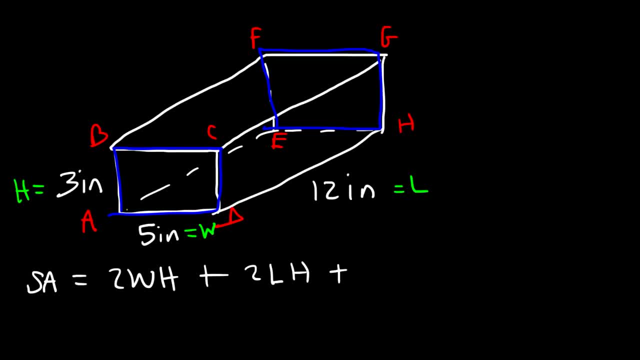 And then we have the face on the bottom ADHE, and also the one on top BCGF, So they have a left L And a width W, So it's going to be L times W but 2LW. 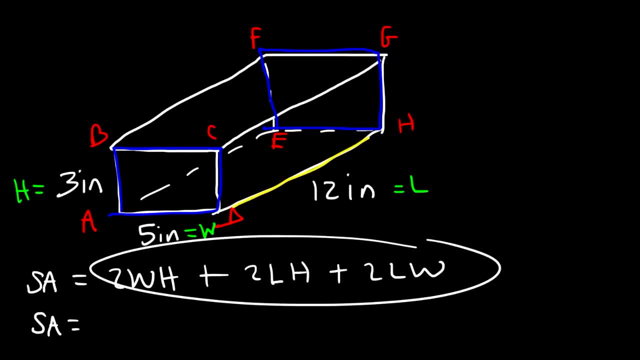 So now that we have the equation, we can find the total surface area. So it's 2WH, or 2 times 5 times 3, plus 2LH, That's 2 times 12 times 3, plus 2LW, 2 times 12 times 5.. 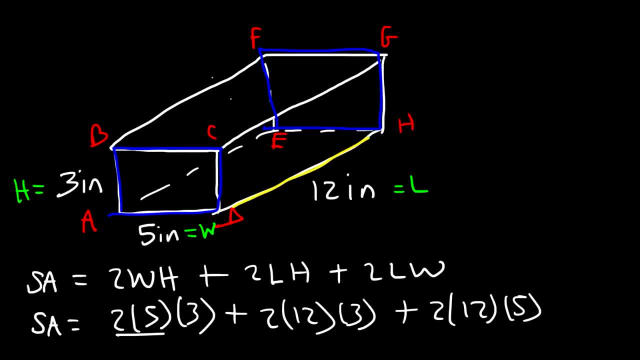 So 2 times 5 is 10, and 10 times 3 is 30.. Now 2 times 3 is 6, and 6 times 12 is 72.. 2 times 5 is 10,, 10 times 12 is 120.. 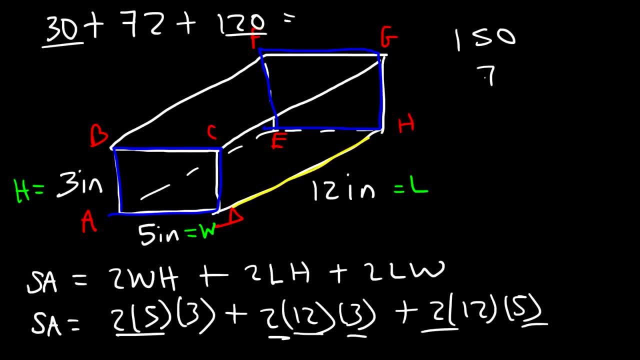 Now 30 plus 120 is 150.. And now let's add 150 with 72.. 5 and 7 is 12.. So total this is going to be 222 square units. So that's the area of this rectangular prism. 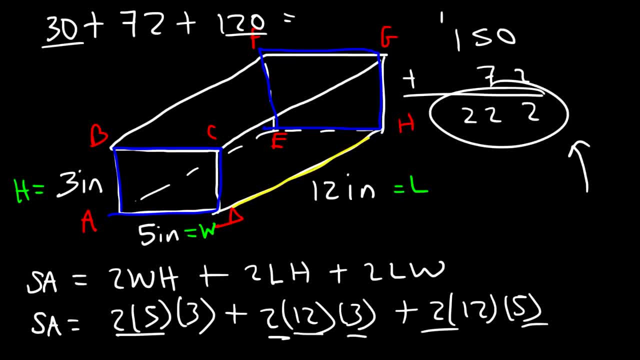 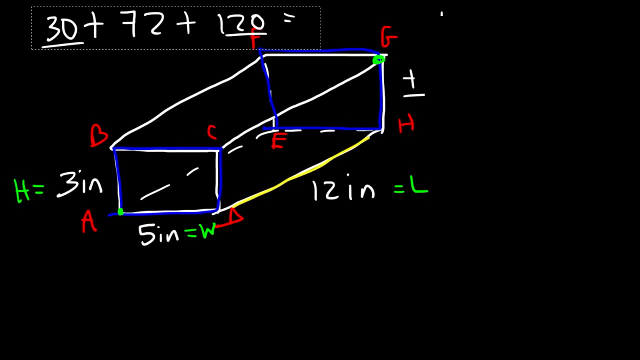 Now here's a separate question for you. If you wanted to calculate the diagonal length between A and G, what would it be? How would you do it? Go ahead and try it, Go ahead and try it. So first, So first. 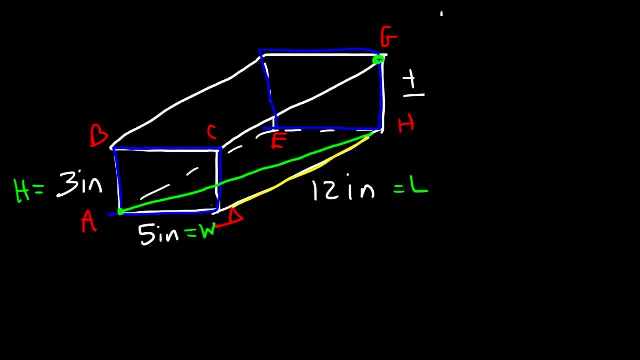 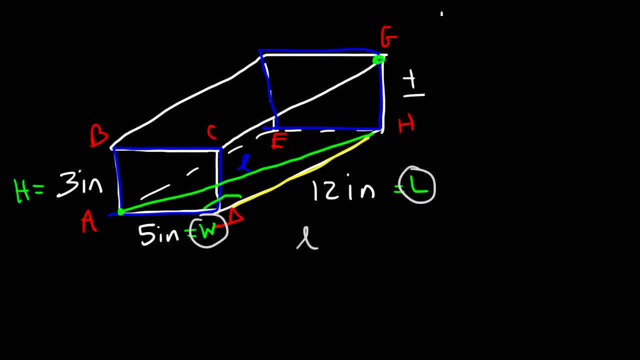 using W and capital L. So lowercase L or L squared is going to be W squared plus capital L squared. Now what we need to do is draw another right triangle- Let me use a different color- Between A, Between A and G. 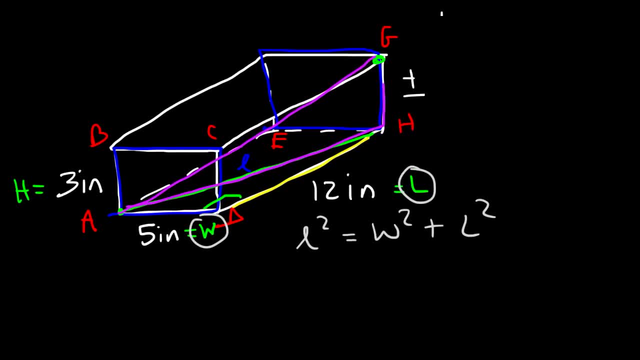 G. So focus on this right triangle that you see here, And let's say that this is the diagonal left D. So D squared is going to be L squared plus this segment which is H, So it's L squared plus H squared. Now I'm going to replace L squared with W squared plus L squared. So 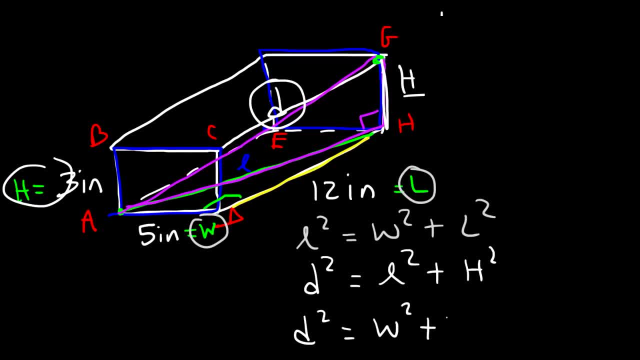 D squared is really W squared plus L squared plus H squared, So that's how you can calculate the length of the diagonal. So D is going to be the square root. that is, if we square root both sides of W squared, which is 5 squared plus L squared, that's 12 squared, And then 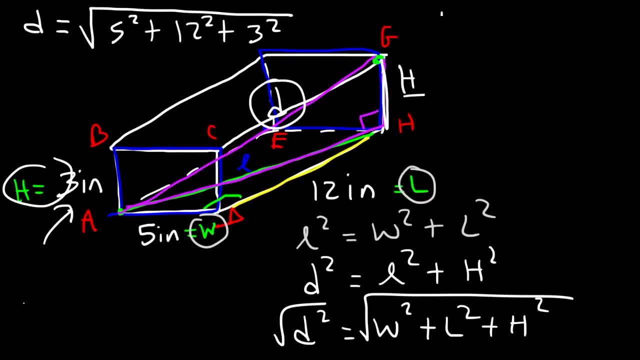 H squared, that's 3 squared. So 5 squared is 25.. 25.. 12 squared is 144.. 3 squared is 9.. 25 plus 144, that's 169.. Plus 9, that's 178.. So D is.